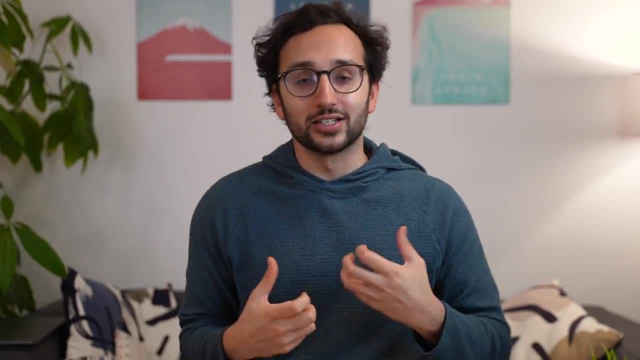 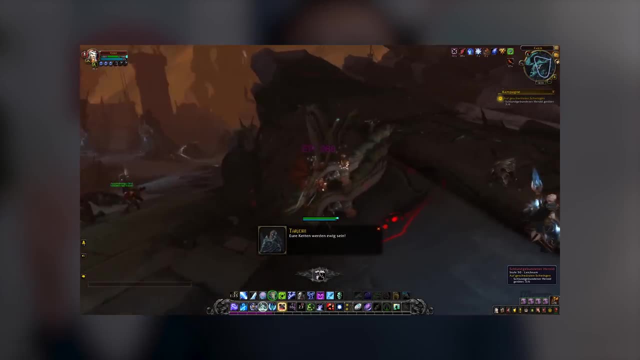 because I was obviously in need of empowerment, And it helped me realize that my time is entirely within my control, Like right now I'm filming this video because I want to be Earlier. today I spent six hours playing World of Warcraft because that's what I wanted to do. 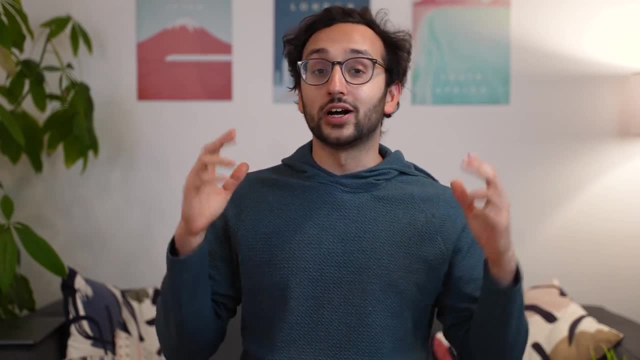 I could not have said I don't have the time to work out today. Instead, it was a case of I'm actively choosing not to make the time to work out today, And so, when it comes to time management, like step one is always to recognize. 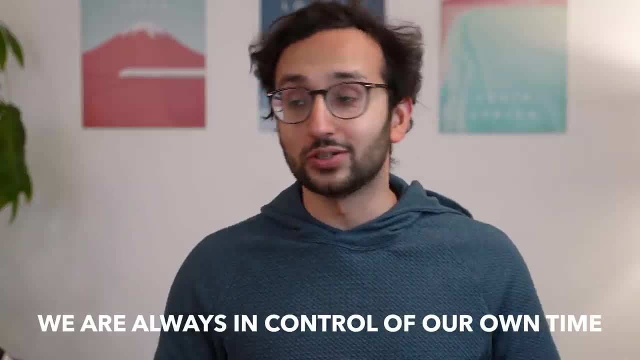 that we are always in control of our own time. Yes, you might have a boss, Yes, you might have parents telling you what to do, but fundamentally you are in control of your own time and you can choose to do whatever you want with that time. 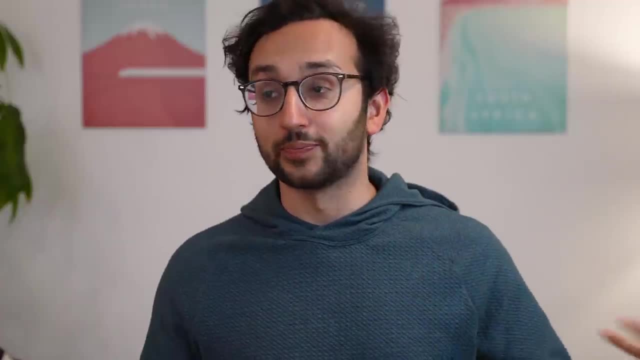 If you don't have the time to do something, that something is just not a priority, which is fine. but don't pretend like the reason you're not doing it is because you genuinely don't have the time. Point number two is the title of this book by Derek Sivers. 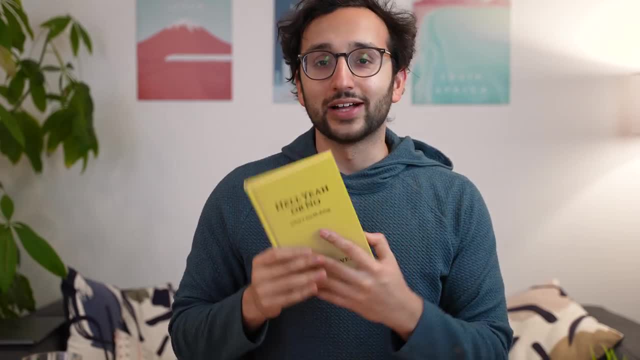 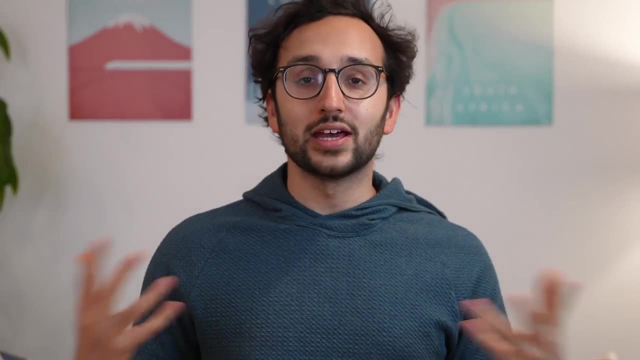 "'Hell Yeah or No, What's Worth Doing". Now the vibe here: hell yeah or no. it kind of says it all in the title. When we're young and we don't have very many opportunities in our lives, we should probably say yes to the majority of things. 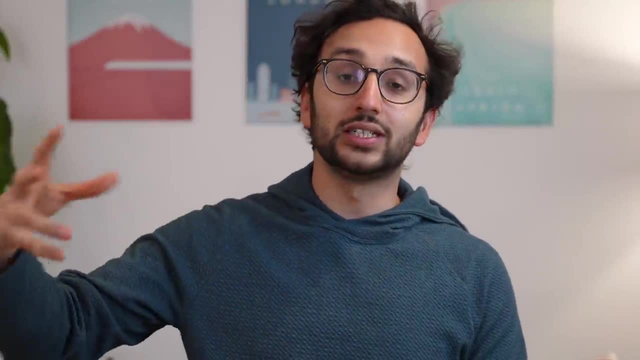 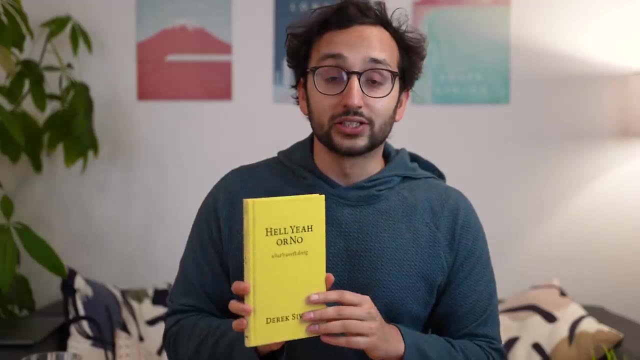 that are coming our way, But as soon as we get to a point where we're starting to get more inbound leads than we have time available, we start operating with a hell yeah or no maxim, And the idea there is something is either a hell yes 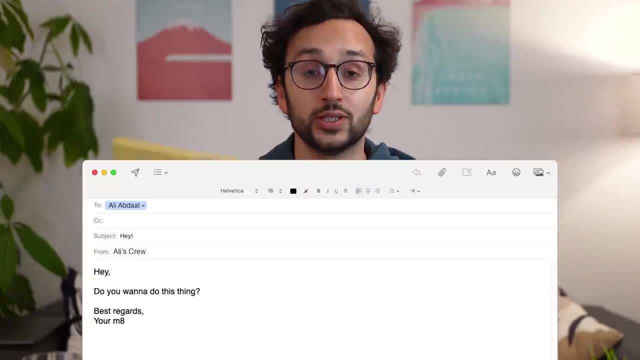 or it's a no. And so if I get an email from someone saying "'Hey, do you wanna do this thing' And I'm thinking maybe it sounds kind of all right, then my default position is gonna be no. If I get an email from someone saying 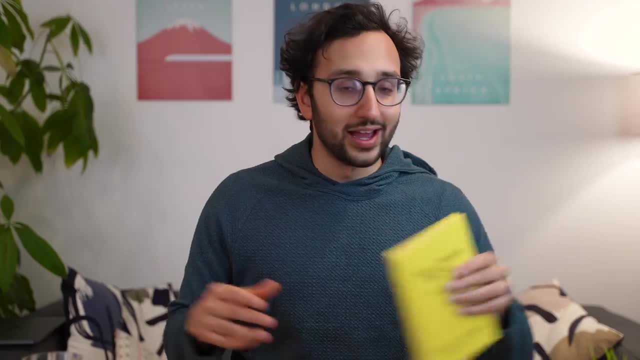 "'Hey, do you wanna do this thing' And I'm like hell, yeah, then I'm gonna do the thing. And I'm trying to get better at using this principle in my life, because even now, my calendar is full of a lot of things. 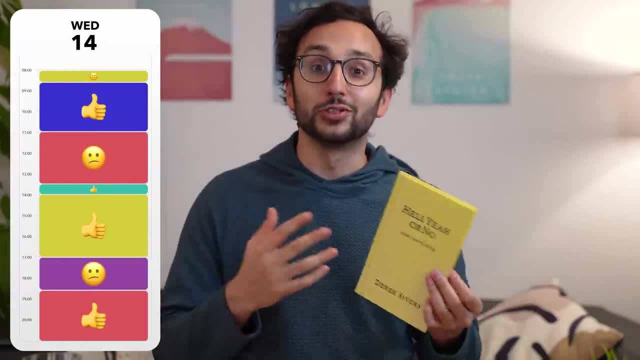 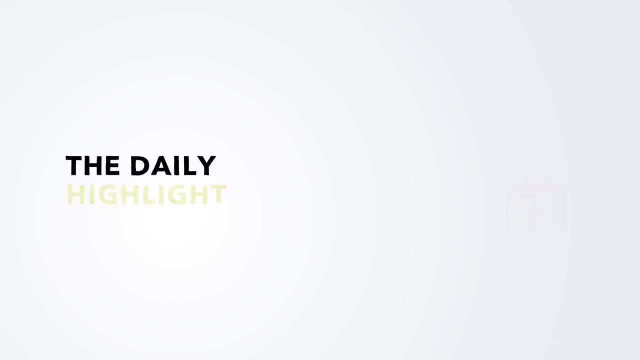 where I'm like oh yeah kind of, rather than hell yeah too, And I always regret doing it when it comes down". So hell yeah or no, just like. learning to be okay with saying no to stuff is another really important principle of time management. 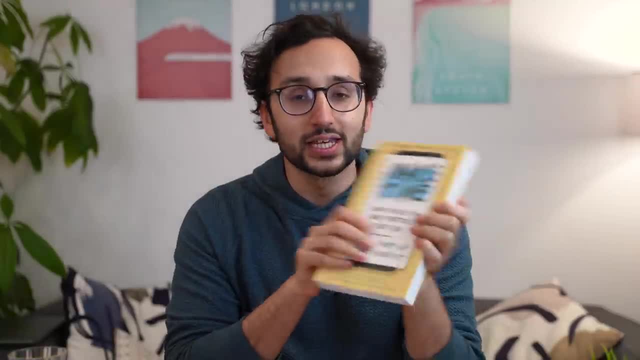 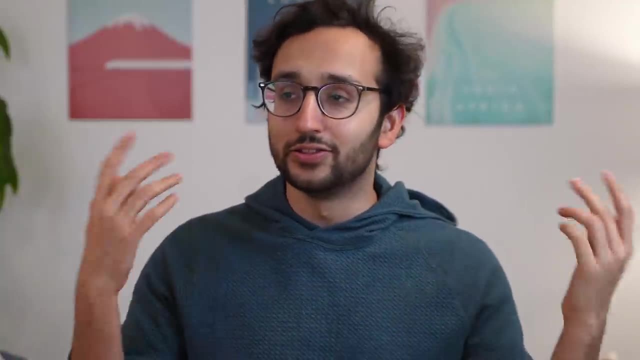 Thirdly, there's a tip I picked up from this book called Make Time by Jake Knapp and John Zeratsky, And this tip is called the daily highlight. This is like deviously simple. Basically, the idea is that every day we decide this thing. 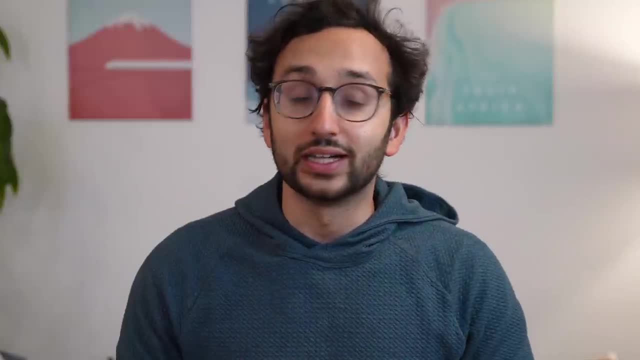 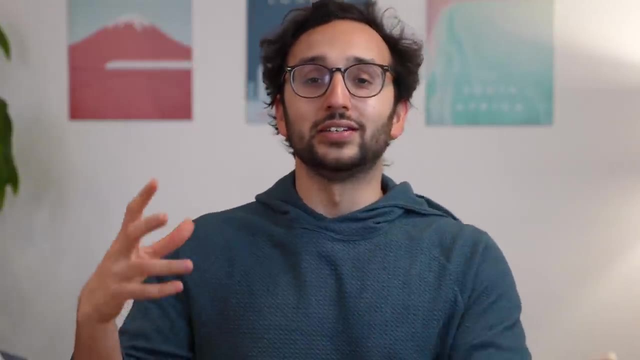 this one thing is gonna be my highlight of the day. This is the only thing I need to get done today And on the days where I set a daily highlight- and I try and do this every day- I always get the thing done and I'm always really happy at the end of the day. 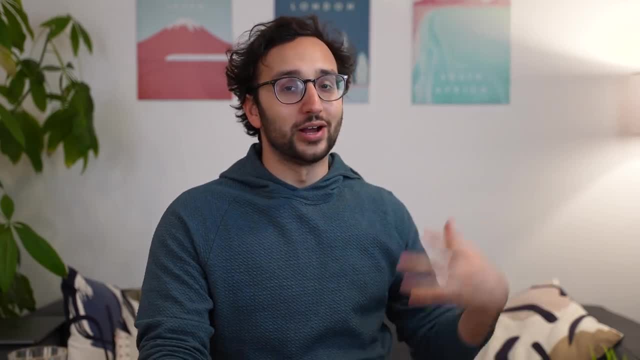 But if I have a day where I don't set my daily highlight, then I kind of drown in my to-do list and I have this just image in my head of like oh yeah, I need to do this and this and this and that. 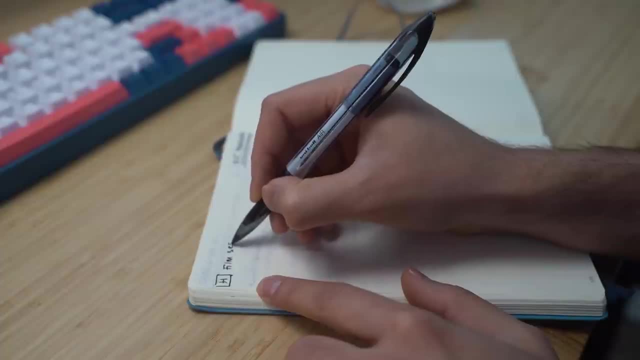 And it's a lot harder to get stuff done, Whereas on days where I have the daily highlight, I have that just one thing that I'm focusing on. You know, this is the most urgent or the most satisfying or the most fun thing I have to do today. 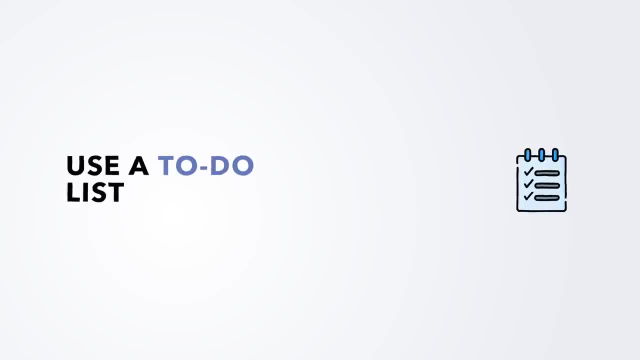 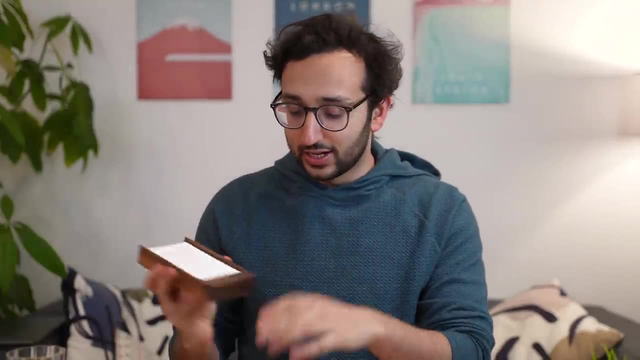 And then it just really, really helps with my time management. Tip number four for time management is to use a to-do list, And these days I use a physical to-do list with this Analogue by Ugmonk. It's very nice. 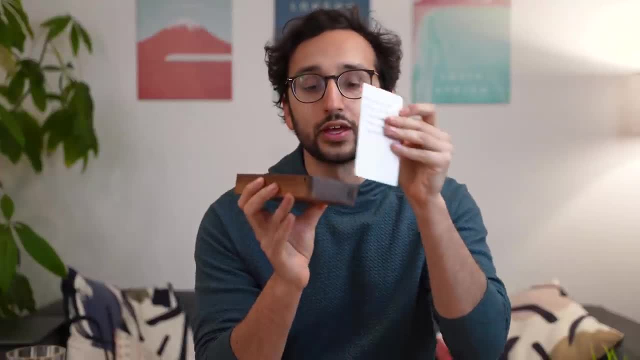 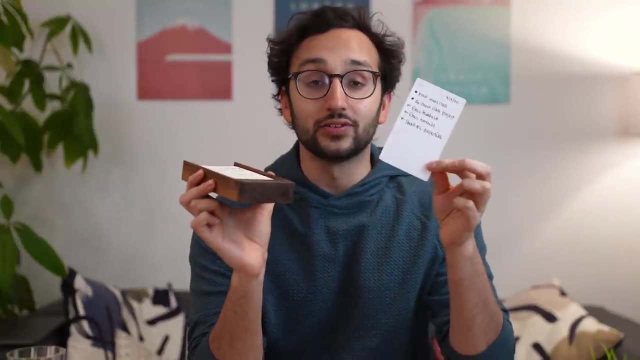 It's like you get these like note cards and then you get this like wooden thing and you like put the note card in the thing and it looks like this: And that means like every morning, once I figured out what my daily highlight is, I make a list of the other stuff that I have to do that day. 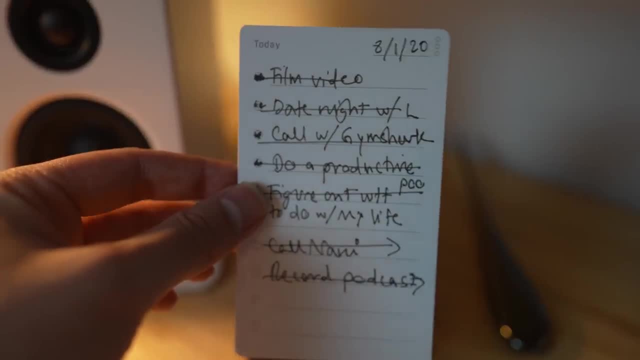 and I shove it on a list and then I tick them off and cross them off with physical pen as I go throughout my day. It doesn't really matter what system you use for a to-do list, But again there's a general principle of productivity. 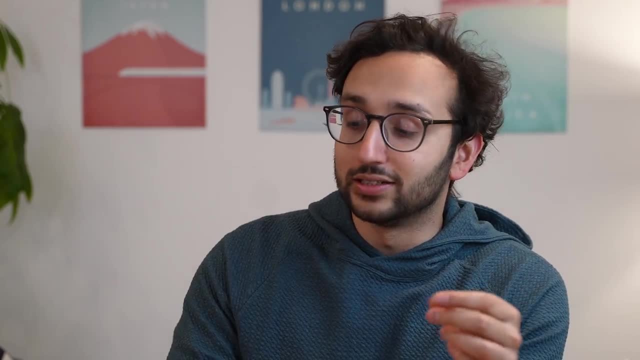 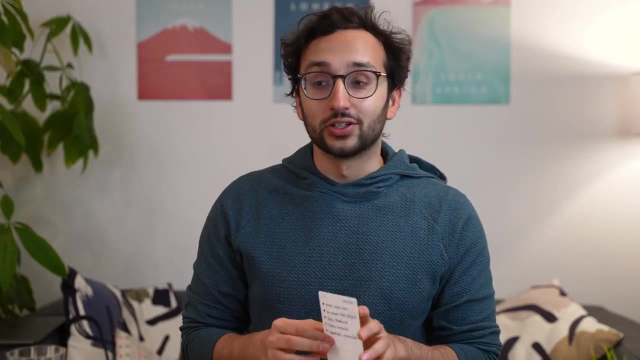 which is that our brain is for having ideas, not for holding them, And a big part of why we let stuff slip through the cracks when it comes to managing our time and managing our productivity is because we haven't written them down, And so anytime I need to do something, 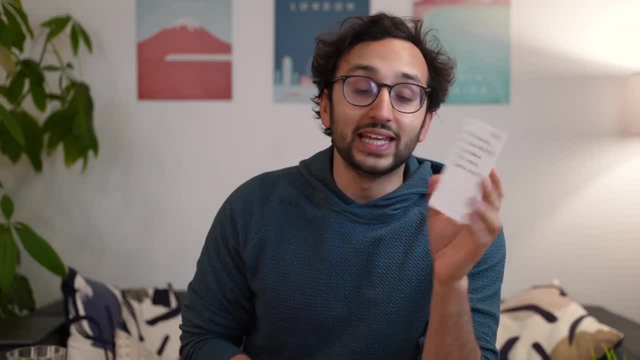 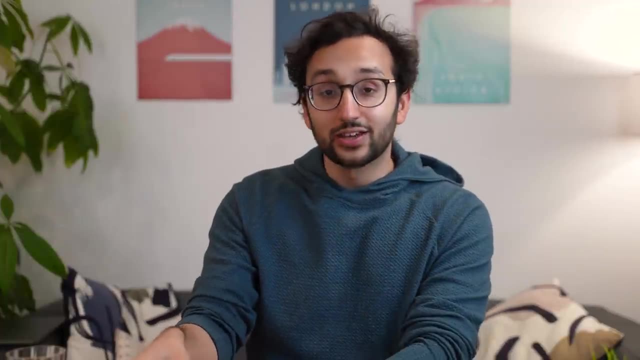 I write it down into an app- These days I use Roam- But then when I figure out my daily to-do list, it's all based on this Analogue system by Ugmonk, which is very nice, And it's kind of cool having a physical to-do list. 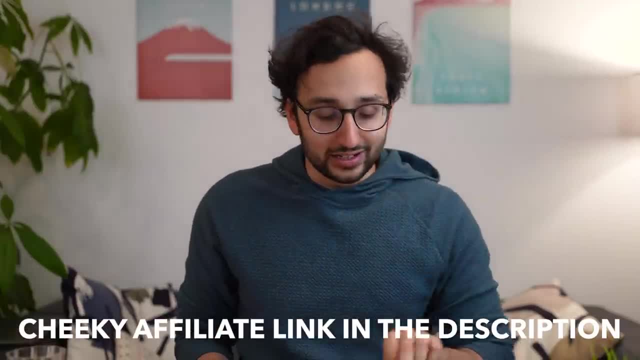 in front of me that I can cross things off of and it just feels nice. And yeah, even at work, when I'm working as a doctor, I use physical to-do lists to manage my patient list, to manage my list of tasks. 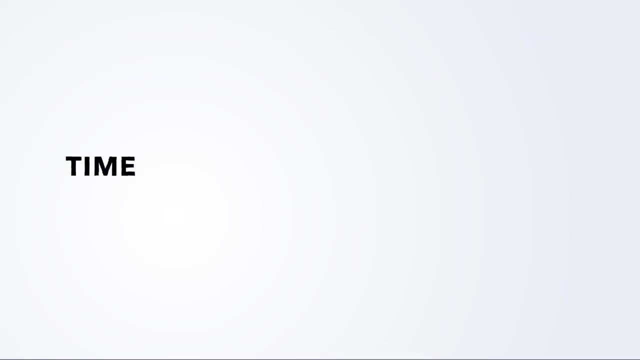 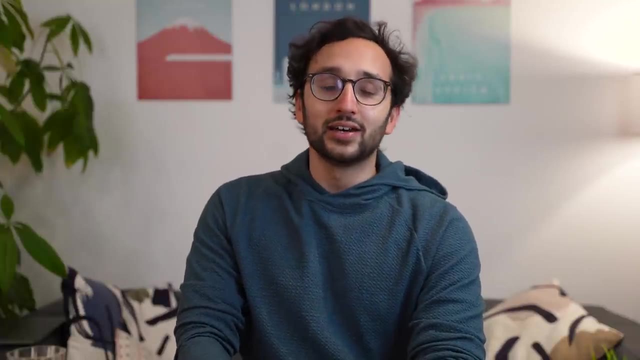 There's something incredibly satisfying about crossing something off which you just don't get when you use an app. Principle number five for time management is the concept of time blocking. Apparently, this is something that Elon Musk does all the time And basically the idea there is. 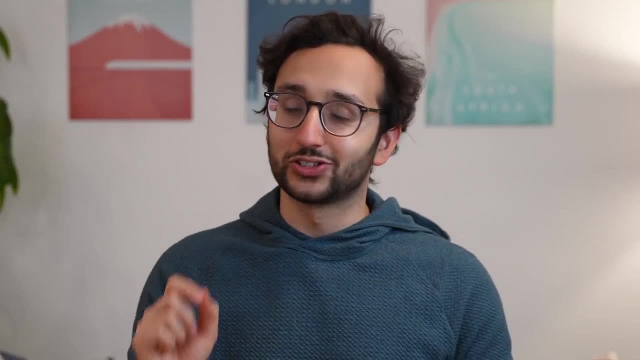 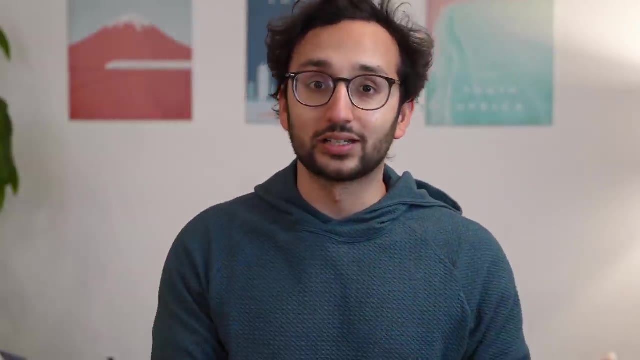 anytime we need to do something, we put a block for it in our calendar. So I don't like doing this for absolutely everything, because I'm a bit of a waste man And I think the more time I spend managing my productivity system, the less time I spend actually getting stuff done. 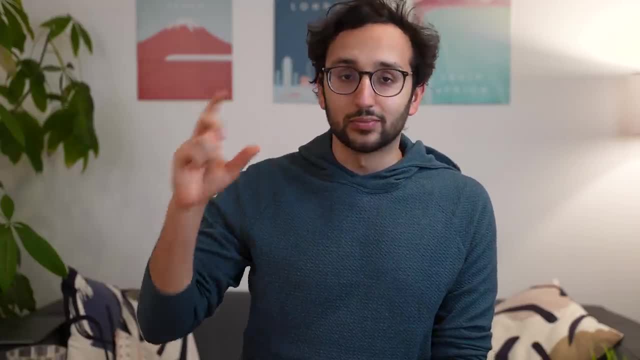 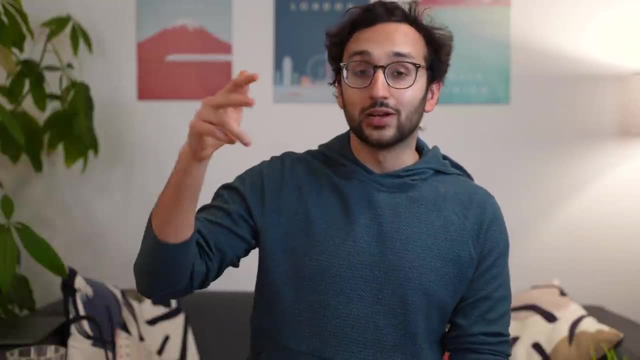 and then it's just all completely pointless. But the one thing that I always schedule into my calendar at the start of the day is my daily highlight. So if I've decided, my daily highlight is filming this video. usually well, I'll try my best. 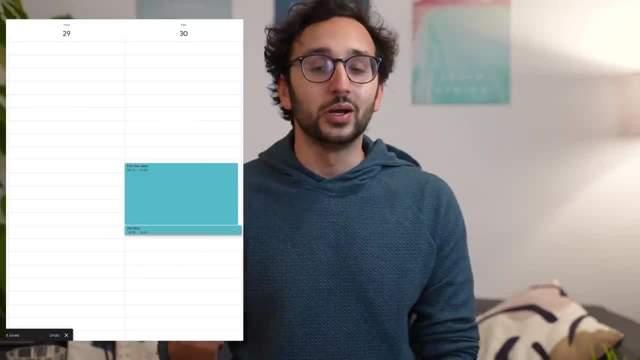 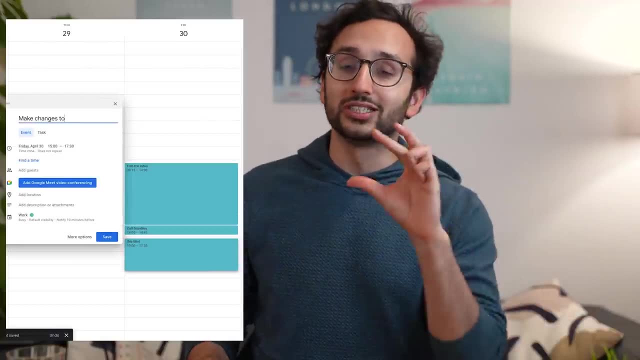 to schedule it into my calendar at the time where I know I'm gonna film the video. If my daily highlight is call my grandma, I will literally schedule it into my calendar. If my daily highlight is make changes to my website, I will schedule it at like for a block in my calendar. 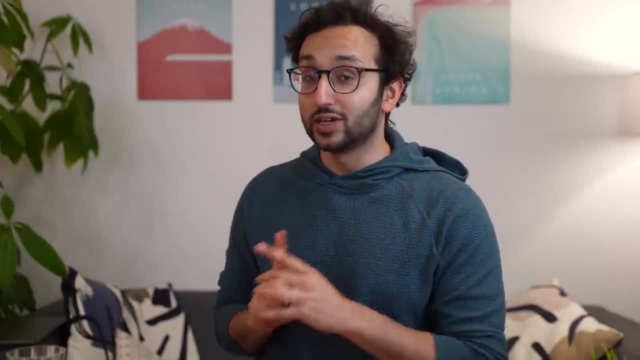 And that's like really nice and reassuring because it means that that one thing that I've decided is really, really important is always gonna get done because it's always on the schedule And then if I need to move it around, I'll move it around if something comes up. 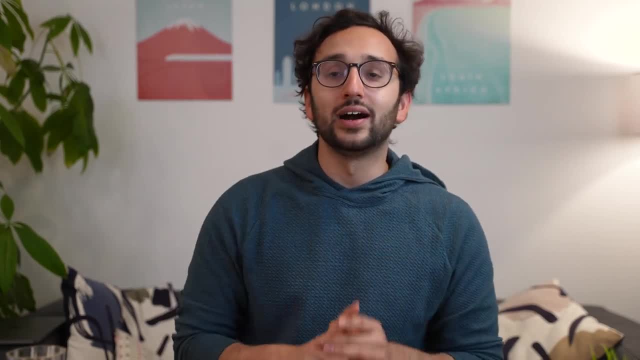 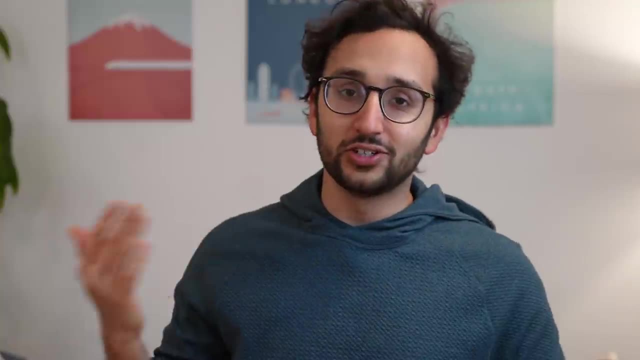 but at least it's there on the schedule by default. And this thing where you combine the daily highlight with time blocking it in the calendar is just incredibly useful. Everyone always kind of thinks that like, oh, but only one thing a day, don't you have to do more than that? 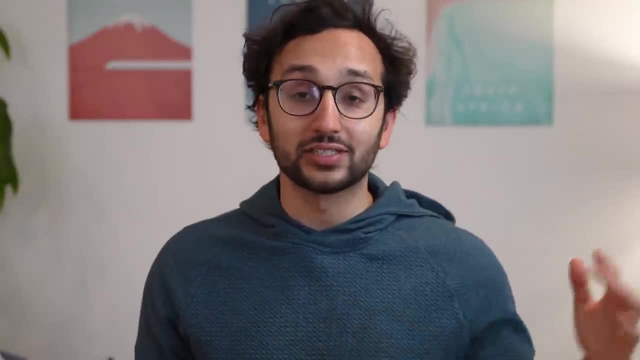 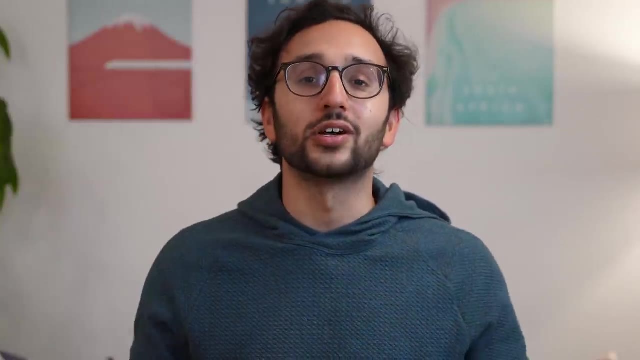 And yeah, you do kind of have to do more than that in most of our lives. But imagine if every single day for the next year, you could actually do the one thing, the one most important thing to do, that day you'd make a hell of a lot of progress. 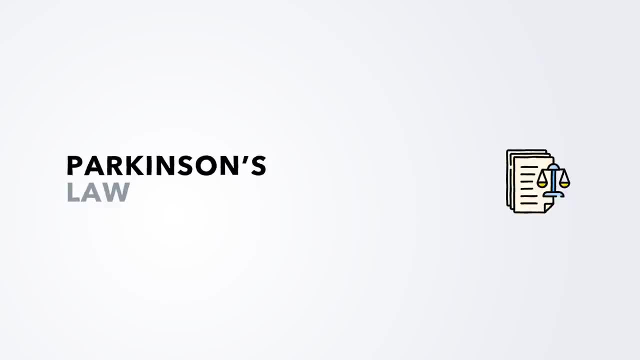 over the course of the year, and it would just be absolutely game changing. Principle number six is related to something called Parkinson's law, which is that work expands to fill the time that we allocate to it. So if I have to film a YouTube video in a day, 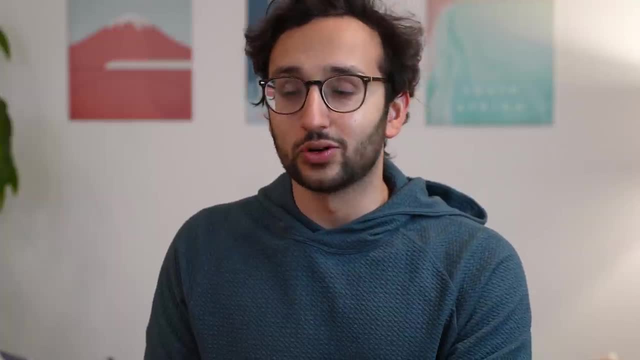 and I give myself the whole day to film that YouTube video, inevitably it's gonna take all day to film the YouTube video, Whereas if I only give myself half an hour or an hour to film the YouTube video and I fill my day up with other things, 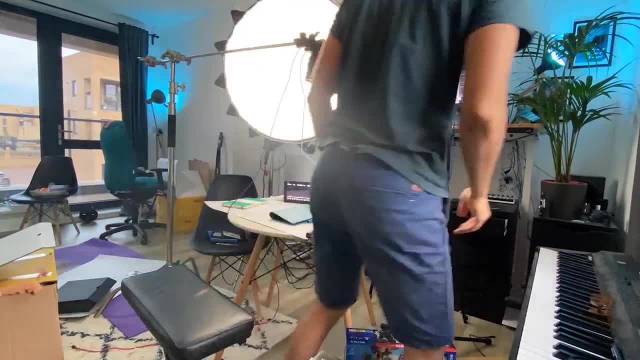 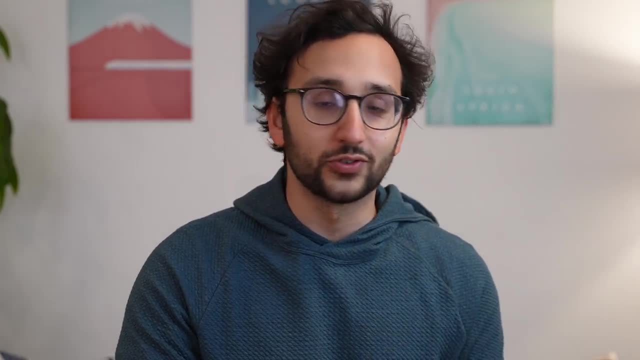 then inevitably, I get the video done in that small amount of time, And so the actionable advice here is to leverage artificial deadlines, even when it's something like filming a new course. like you know, I'm working on a course for YouTube for beginners. 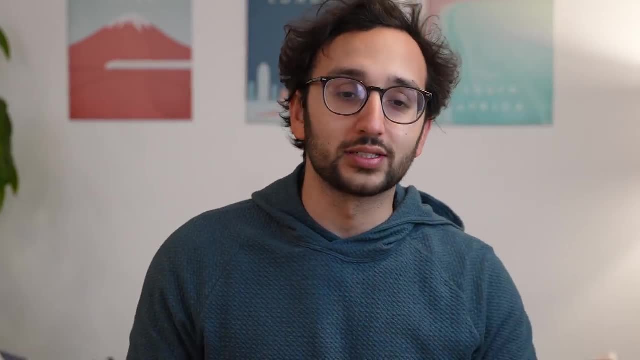 where I kind of film and talk you to everything about my YouTube videos, do a production process And this doesn't really have a deadline, Like I could literally do it whenever I want. I don't have to do it, It's purely optional project. 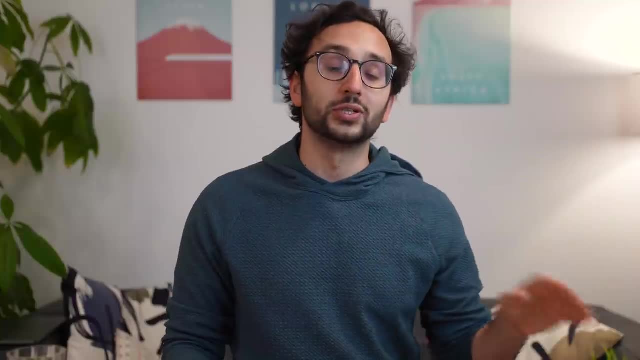 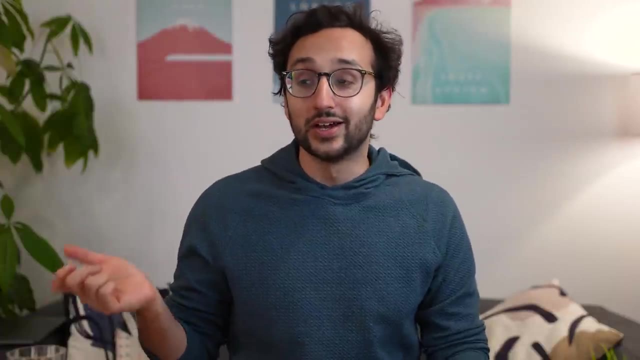 but I've set myself the goal that, okay, you know what I'm gonna film all of this course next weekend And I've blocked out time in my calendar next weekend to film the course And that's an artificial deadline, which means the course is gonna get done. 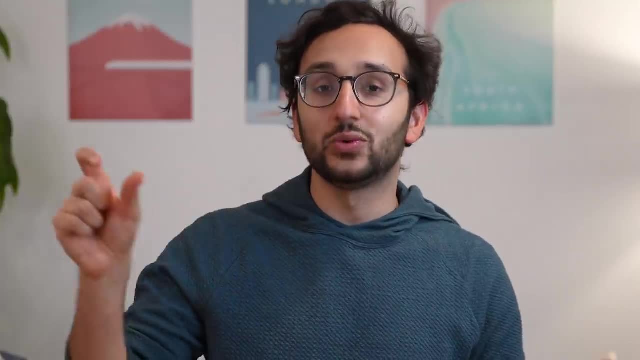 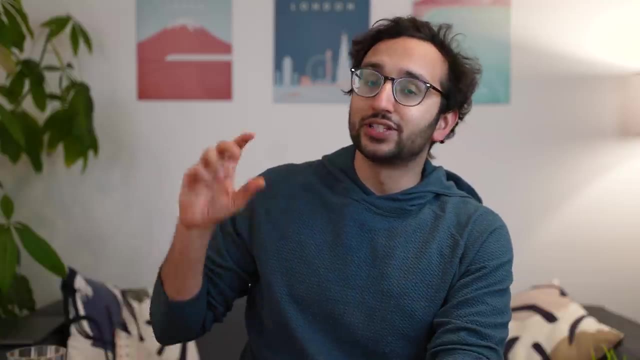 Whereas if I just had it in my mind or in my to-do list, without a deadline, without a schedule, it would just inevitably never, ever get done. Point number seven is one I've started applying recently, and that is having protected time When you are an entrepreneur. 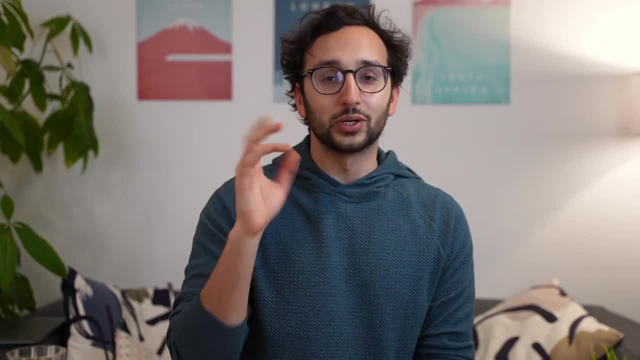 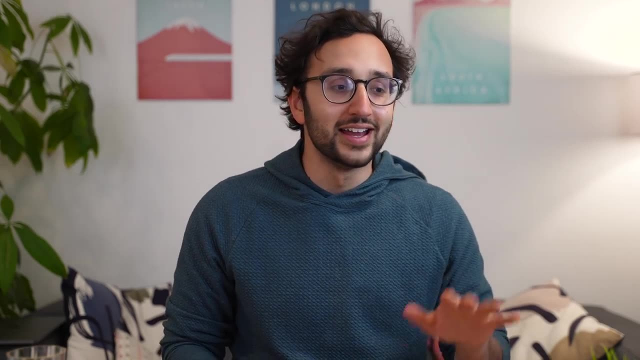 and you're like working for yourself and all that kind of stuff, you end up basically being able to set whatever schedule you want. But, like, if you're like me and you're like making connections and making friends with people all around the internet, you get to a point where your day is filled. 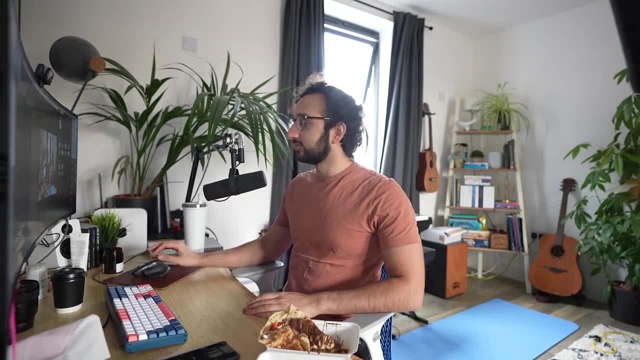 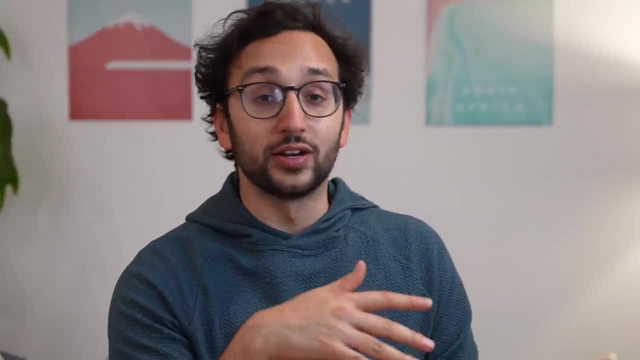 with lots and lots of Zoom calls And I realized that for me, I need to keep my mornings completely free of any obligations or any Zoom calls. And this has been an absolute game changer, because in the morning that means I can wake up whenever I want. 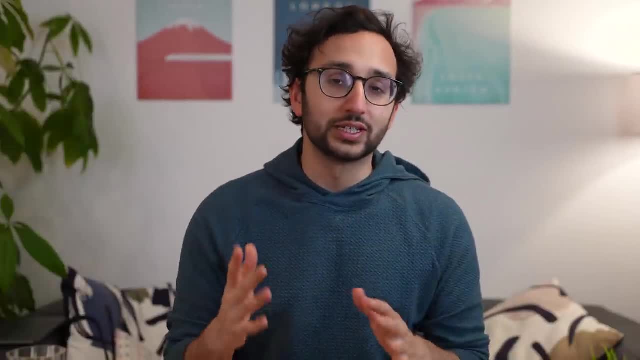 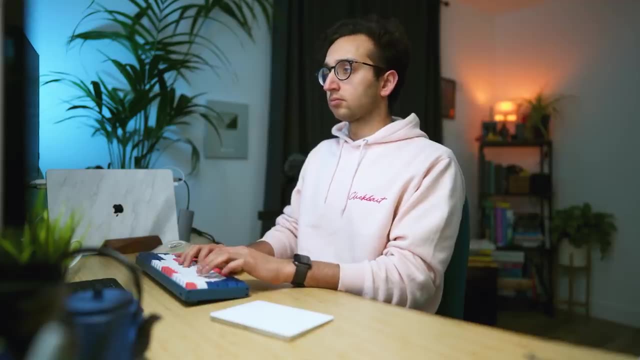 Usually it's half past eight these days, And it means that for a solid like four hours at least I've got uninterrupted time where I can do whatever I want. So these days I'm working on writing my book, And so the morning is my protected time for writing. 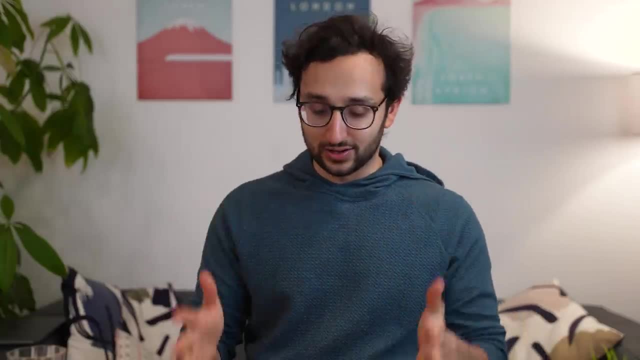 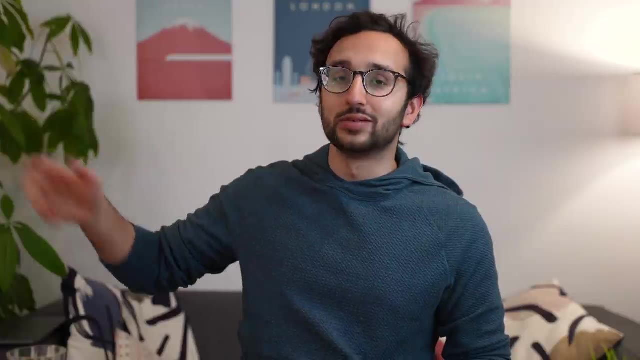 But even on days where I'm not working on the book, it's just genuinely so nice to have that like time slot where I can think about the business or plan some more videos or do the things that help move me forward in my work career. 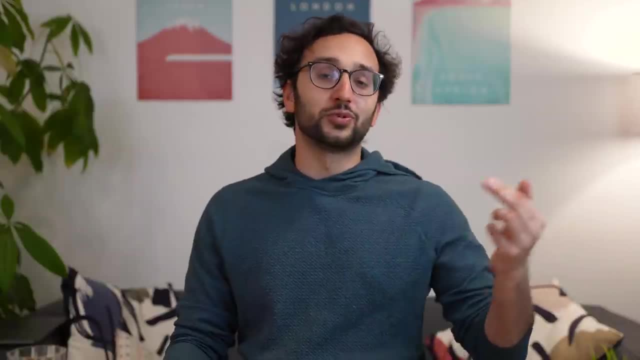 And sometimes, if I'm not really feeling it, I'll just decide. you know what I'm gonna use this protected time to play World of Warcraft or to just kind of relax and read a book on the sofa. So if you're interested in better ways, 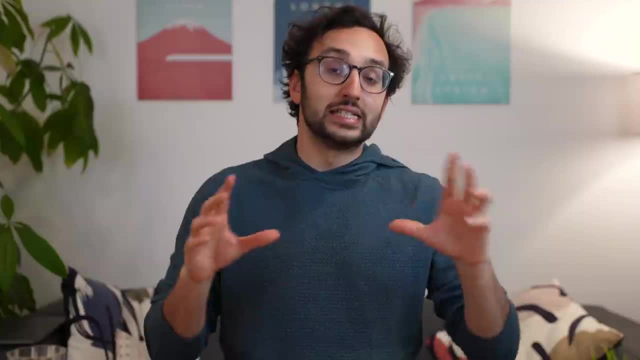 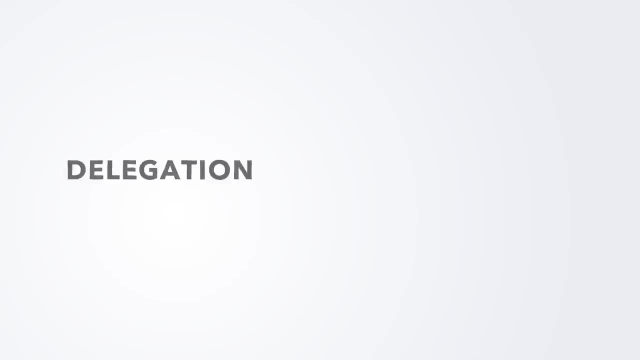 to managing your time, I would recommend figuring out what your protected time is gonna be: Time that is just for you and you alone, or World of Warcraft, and not for anyone else, where no one is allowed to book something in your schedule. All right. principle number eight is delegation. 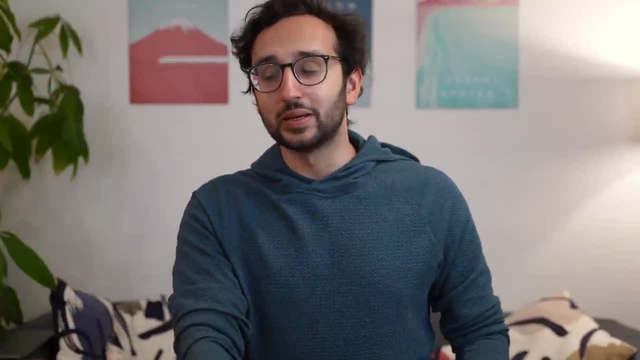 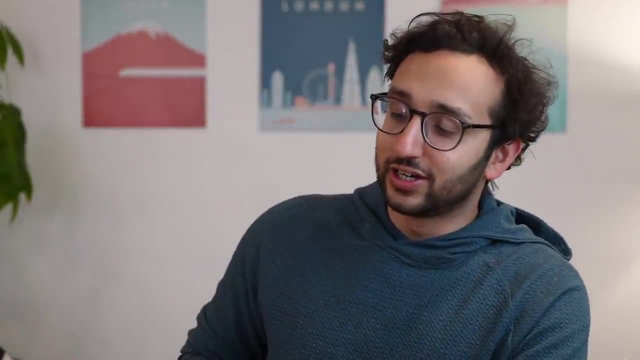 Now this one is a little bit weird, because normally when you say the word delegate, people imagine that, oh well, I can't afford to delegate something, I don't have enough money to delegate to hire someone, And sure, that's probably true. 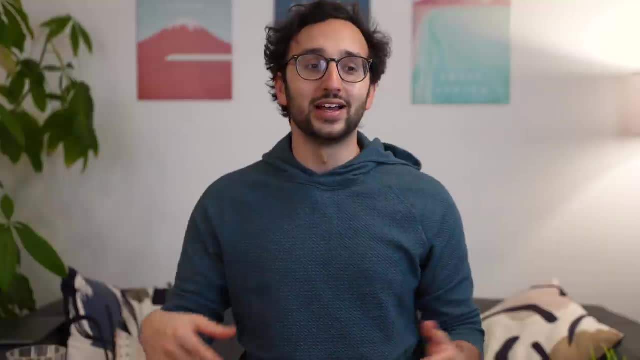 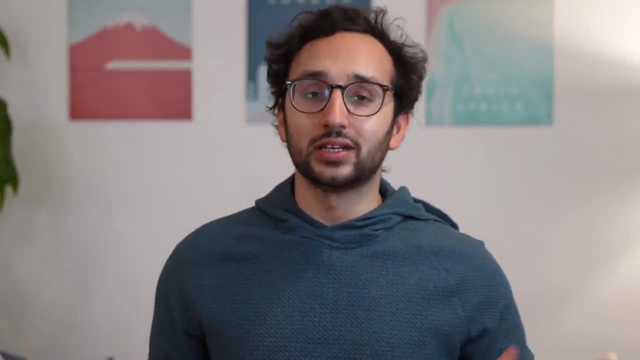 But the way that I think of it, even when this YouTube channel wasn't successful, was that, like, what is actually the dollar value of my time? How much is my time actually worth? And when it came to running my business, I decided that, okay, my time is worth 20 pounds an hour. 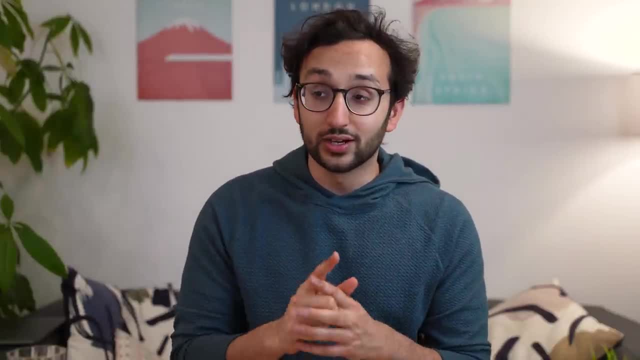 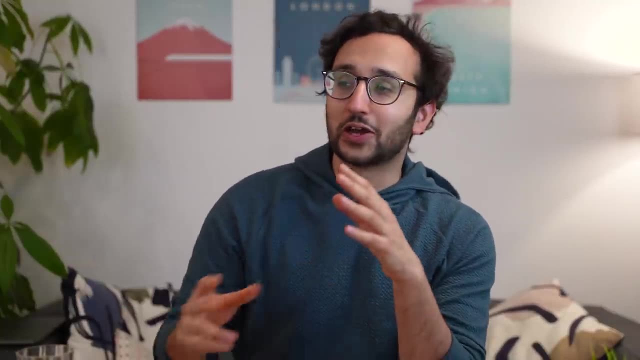 or $25 an hour, And that means that anything I'm doing that I don't enjoy, that I can outsource to someone that I can delegate for less than $25 an hour. I absolutely should do that, And that principle of delegation has encouraged me. 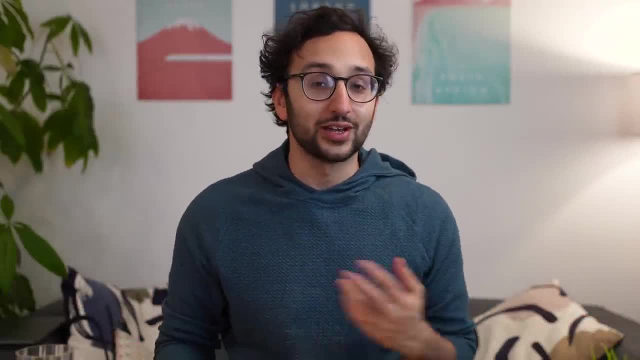 to get a cleaner, which has been great, because now we have someone who comes in to clean the house every other week, which means I don't have to do it myself. And back in the day when I was building my businesses from the ground up. 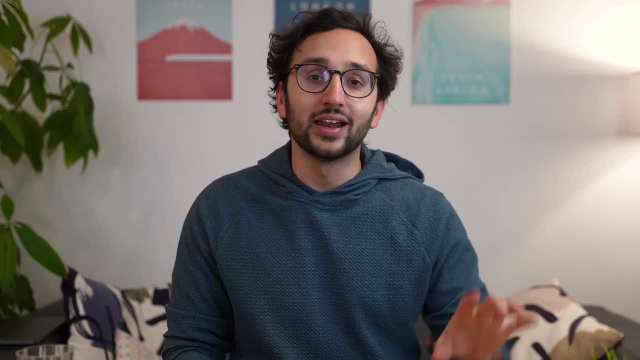 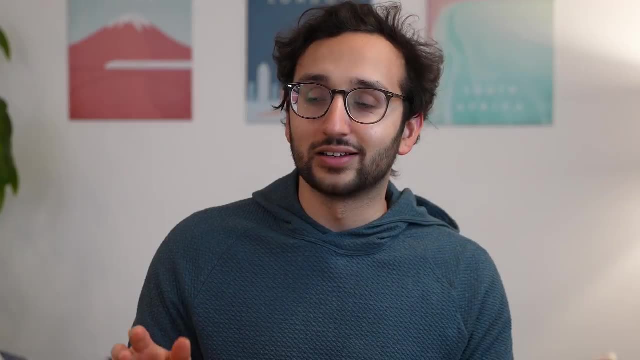 and there was lots of things that needed to be done, like data entry or things like that. I was able to delegate those to freelancers in like the Philippines or in Bangladesh or in India through upworkcom or fiverrcom And like paying them like $7 an hour. 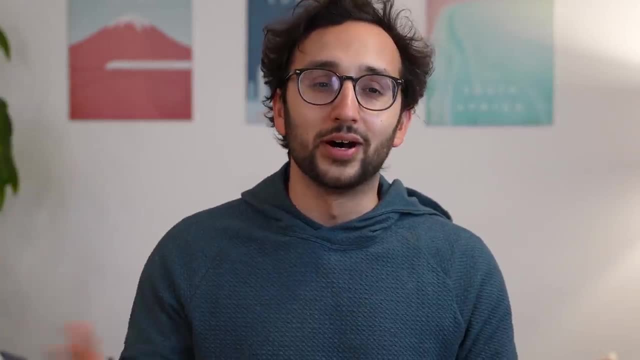 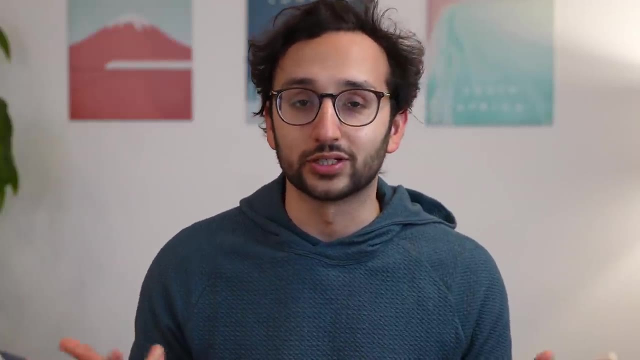 is an amazing like wage for someone for work in the Philippines, But it was fantastic for me because it freed up my time to do things that were adding more value to the business and to my life than doing data entry, for example, And so, whatever your circumstances are, 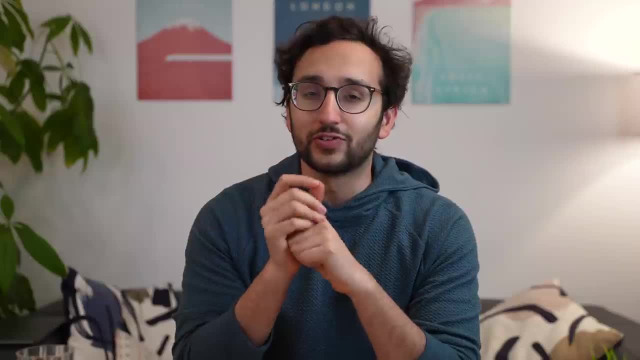 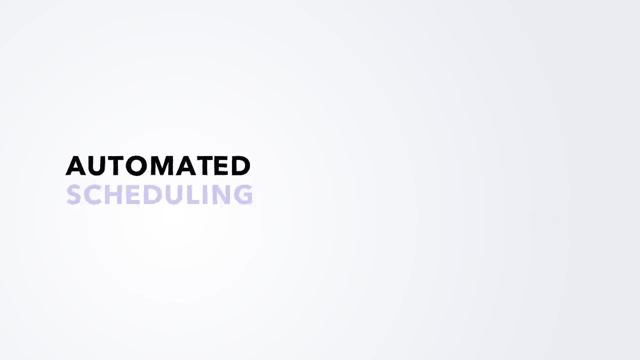 I'd encourage you to think about what is the dollar value of your time And potentially, if you want, can you delegate stuff that's cheaper than that to other people. Potentially, Tip number nine for time management is to try and automate scheduling as much as possible. 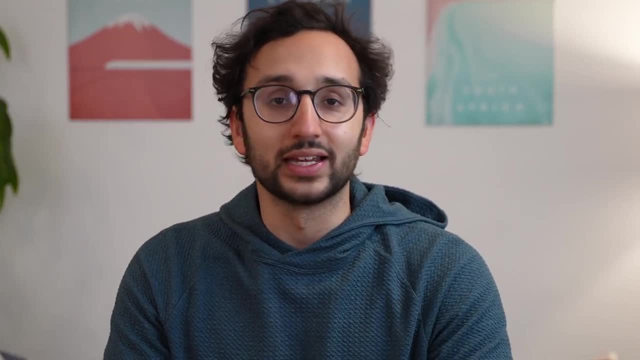 Now that we're in the world of like Zoom calls and like chatting to people over the internet basically every day, I found I was wasting a lot of time in scheduling back and forth where I'd be like, hey, I wanna talk to you. 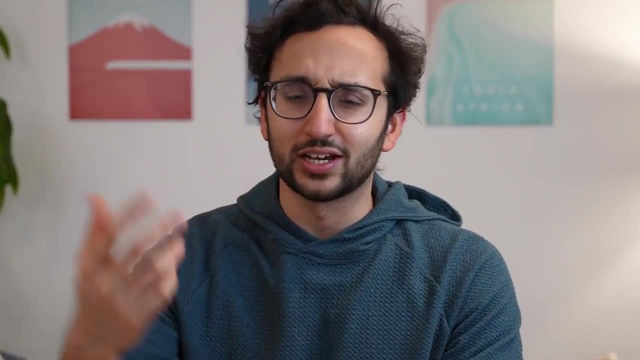 but like: are you free? this time Pacific time, this time Eastern time, this time British standard time, all this kind of stuff, And we'd go back and forth with emails for like a solid 10 days before anything would get done. 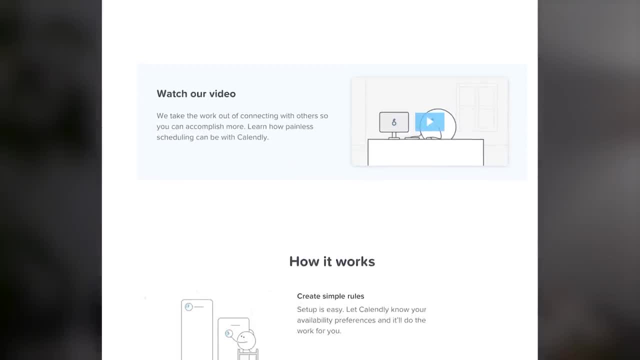 But then I discovered an app called Calendly, and Calendly is great. It's free for. like the free version, I pay for the pro version these days- not sponsoring this video or anything like that, Unfortunately, Calendly. if you're watching this, let me know. 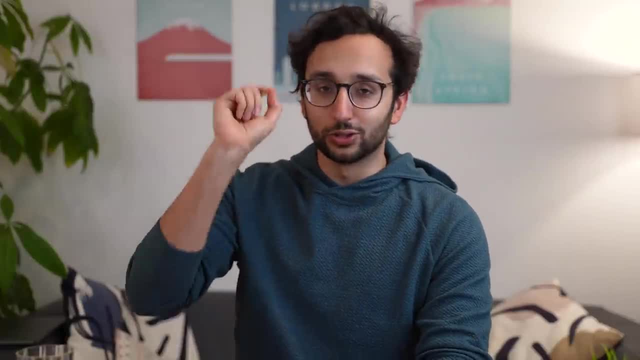 But the idea behind Calendly is you can literally send someone a link and it has like all of your availability and they can just book a slot in your calendar. Now this feels a little bit weird to do initially. it feels like a bit of a power move. 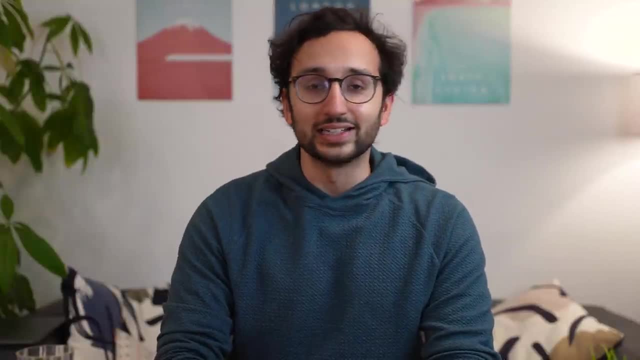 that hey, book a slot on my calendar. But anytime I get a Calendly link from someone, I'm like, oh my God, I'm so grateful because this has literally saved me 20 minutes of my life time that I'm never gonna get back. 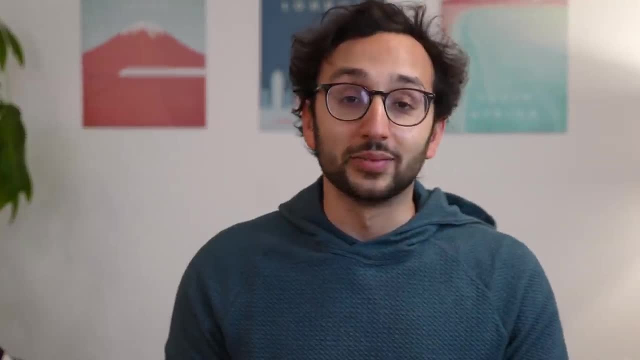 in not having to worry about scheduling back and forth emails. Even sometimes these days, when it comes to like catching up with friends, I just send them a Calendly link and I'm like: look, so, hey man, I'm really sorry. 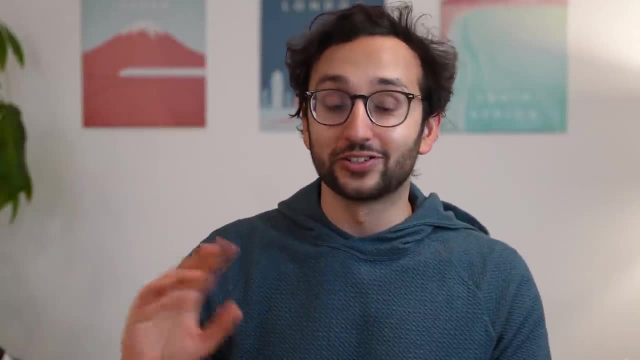 But, like you know, here's a Calendly link. I know we're never gonna talk because the schedules are never gonna align, But if there's a time that works for you, click on this link and he books a time and we have a call and it's nice. 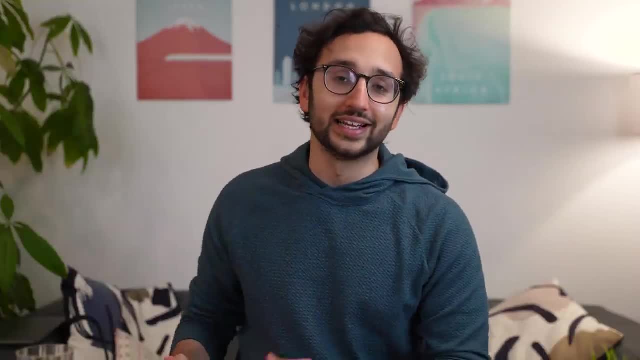 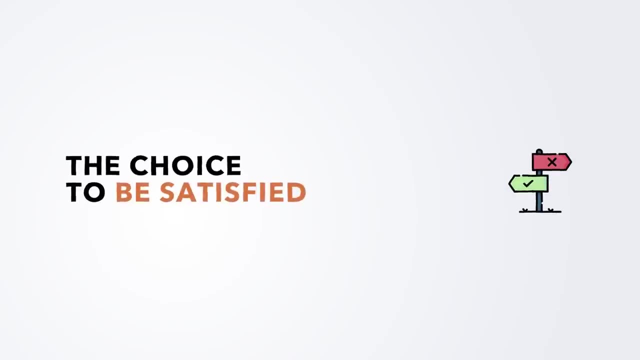 because I've caught up with so many more friends in the last few months through using Calendly links than I did in the last, like three years, of having to schedule back and forth with WhatsApp messages. And finally, principle number 10 for time management. 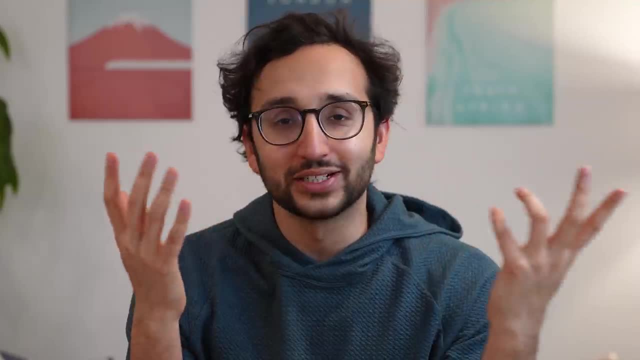 And this is something I've only recently started to appreciate, which is that, like when you're like a productivity nerd and you're interested in like efficiency and getting more done, it's very easy for us to get to the end of the day and to just feel.